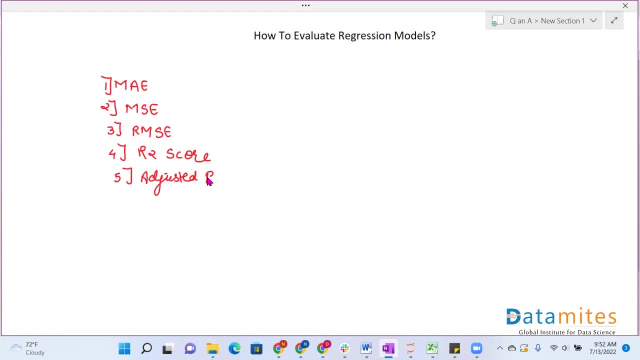 R2 score. So M-A-E stands for mean. M-A-E stands for absolute error. M-S-E stands for mean squared error. R-M-S-E stands for root mean squared error. So let's understand these One by one. 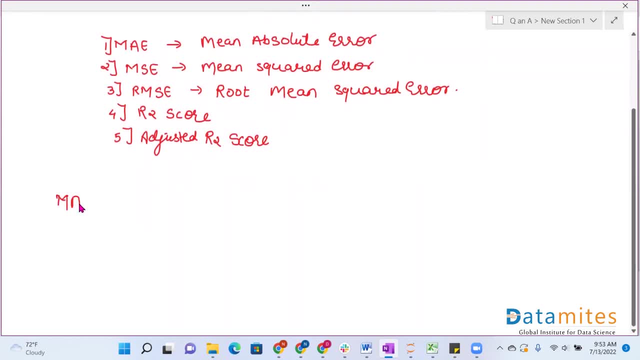 Okay, So let's start with M-A-E. That is mean absolute error. So let's assume that this is our regression line. Okay, So, if this is the data set, my model has predicted, this is data For this data point. my model predicted here: right. 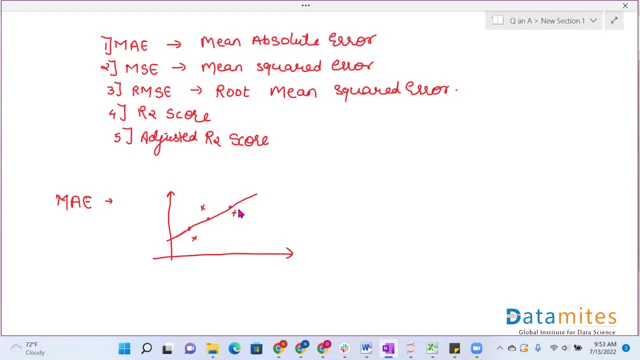 So, whatever will be the data, The data model will predict it on the regression line. Okay, So let's assume that Y1, Y1 is my actual output and Y1 dash is my predicted output. Similarly, Y2 is my actual output and Y2 dash is my predicted output. 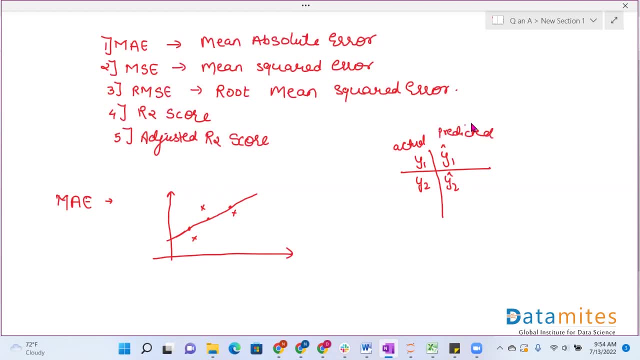 Okay, Okay, So let's assume that Y2 is my actual output and Y2 dash is my predicted output. Okay, So let's assume that Y2 is my actual output and Y2 dash is my predicted output. Okay, So like this, we have these four many data points, right? 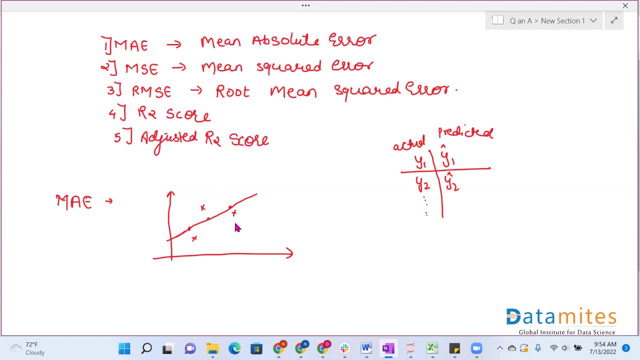 So how will I calculate M-A-E? So mean absolute error is given by the difference between the actual and predicted value. So for Y1, Y1 minus Y predicted, taking the mod plus error for Y2.. That is Y2 minus Y predicted and Y3 minus Y3 minus Y4.. 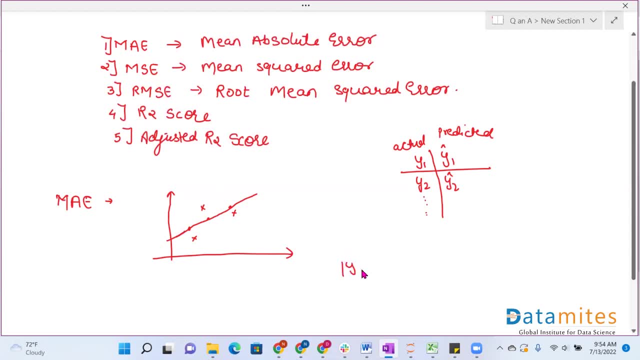 And Y3, minus Y3.. So it means the error is given here. So that is Y2 minus Y predicted and Y4. dash is my predicted output. Okay, So now we know the error. So it is M-M-S-E right. 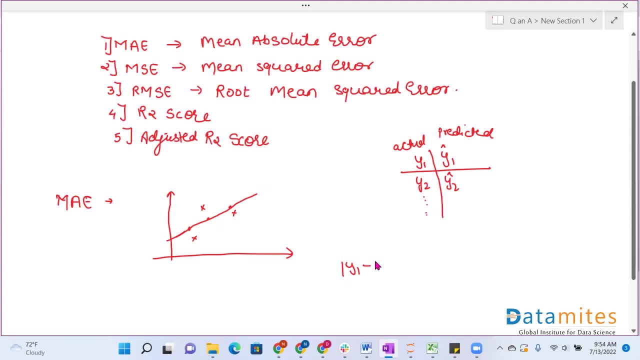 So let's assume that Y2 is my absolute output predicted value. So for y1, y1 minus y predicted, taking the mod plus error. for y2, that is y2 minus y predicted, then y3 minus y3 predicted and up to and data points. 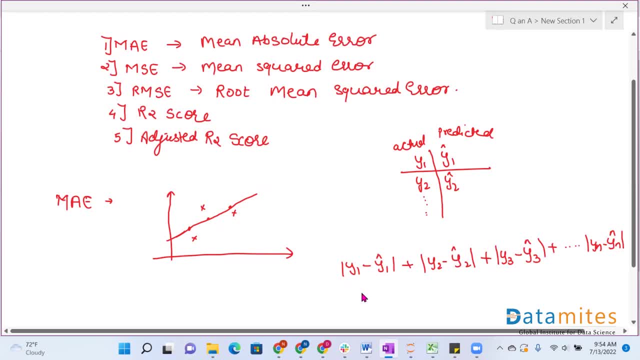 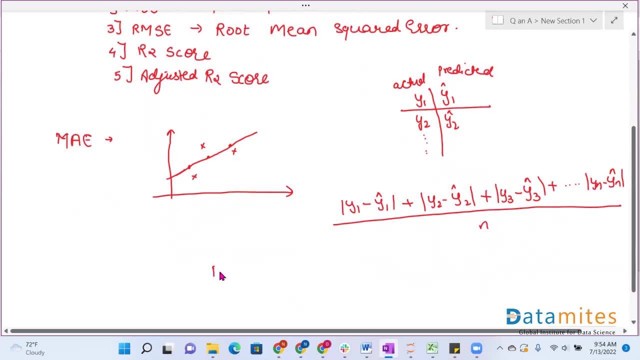 Notice: Okay, So that it is divided by number of data points. So this can be written as: MAE equals to submission of i equals to 1 to n mod yi minus yi hat divided by n. So this is our mean, absolute error. 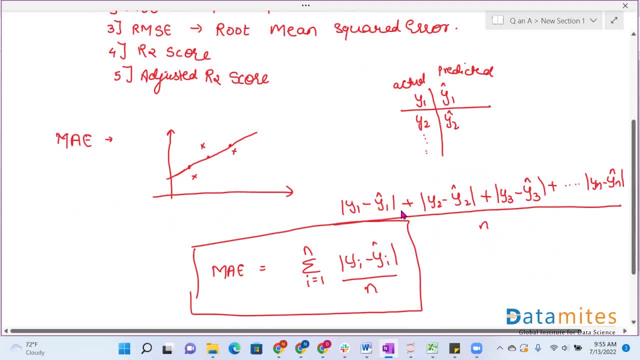 So we will take this as we end this session. So we will take this as we end this session. So we will take this as we end this session: the difference between the actual and predicted value for all the data points, and we will. 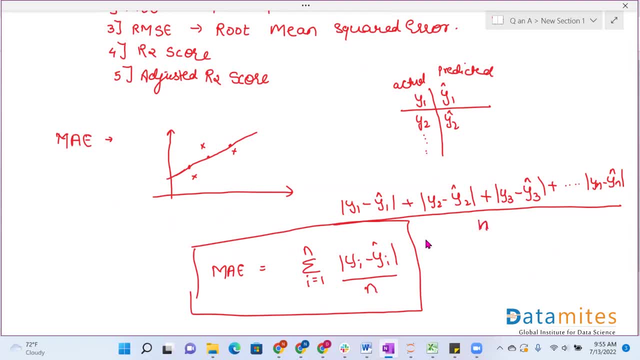 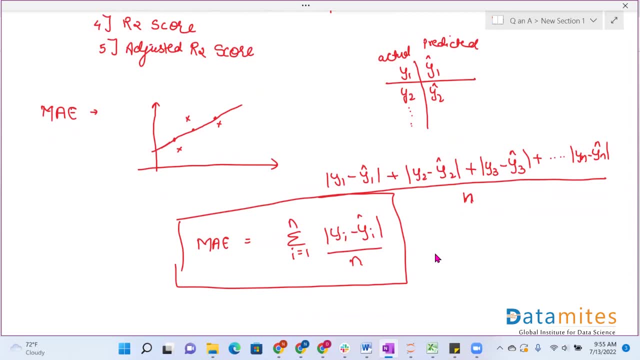 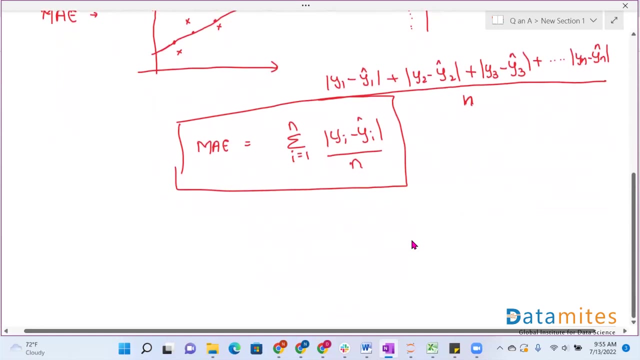 sum it divided by number of data points. that is the mean absolute error. So this is some disadvantage that this is not differentiable and we should. we know that error should be differentiable, So we will move towards the next type of evaluation matrices, that is mean. 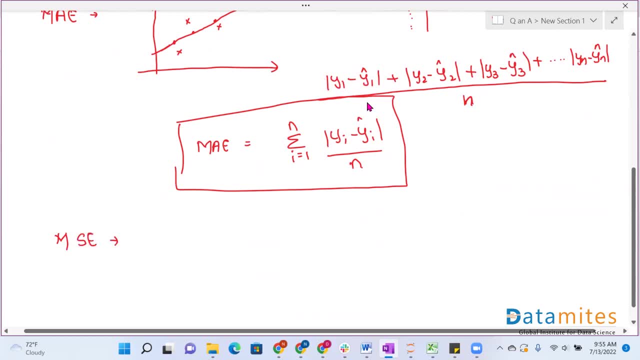 squared error. So here, instead of taking mod, we have square of error. So mean absolute error is given by submission of data points. i equals to 1 to n yi minus yi, hat square divided by n. ok, So in place of mod we have taken square. So in place of mod. on modulus. 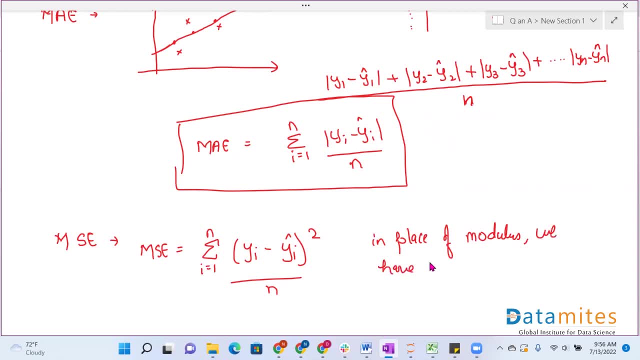 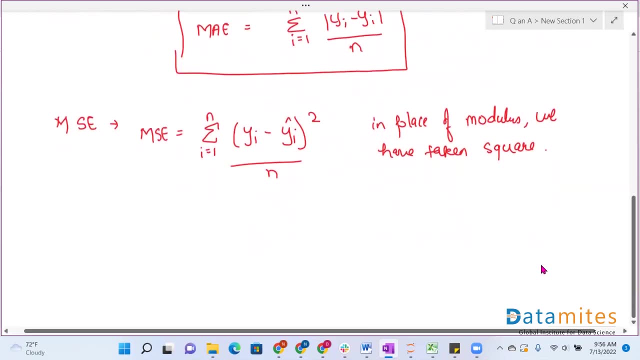 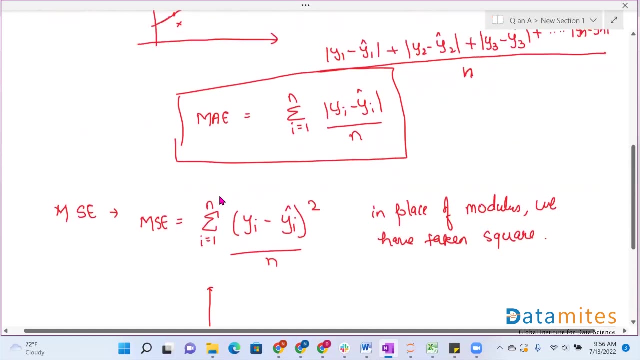 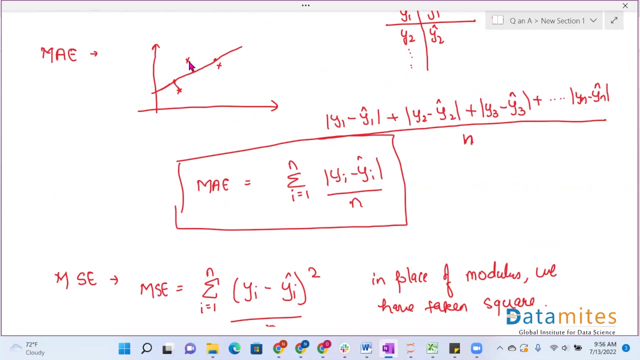 we have taken square of the error. ok, So how we will see this in graph. So here we can see that this is this will take. the difference means this will take the distance, this distance, this will calculate the distance. this is the difference between the actual and predicted. 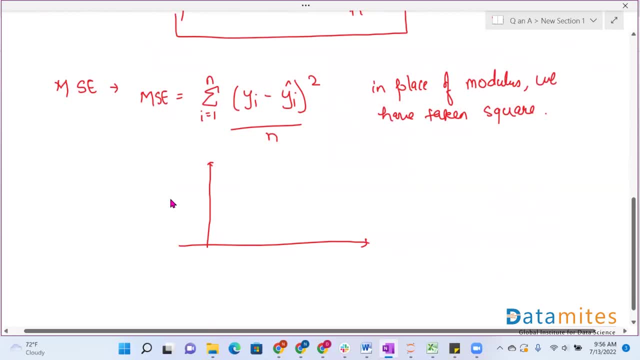 value, But in mean square error, in mean square error. this is our regression line and if this is the actual data point and this is the predicted, So it will take the square. that is area. This for this data point it will take like this. So this, all things will get added. 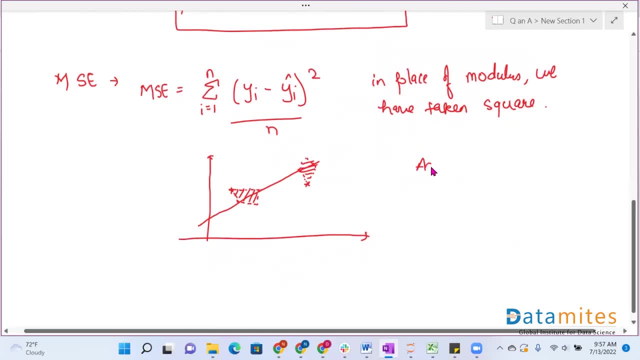 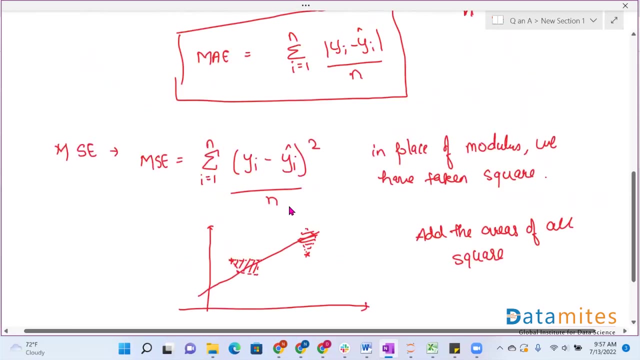 So this will add the areas of all the square. This will add the areas of all square. ok, So the advantage of this is like the disadvantage of MA is covered in MSC, But it has again one disadvantage: that the unit or unit is square. term right: The unit of MSC is square. 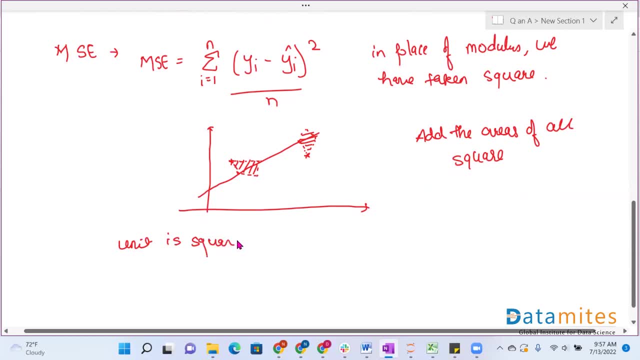 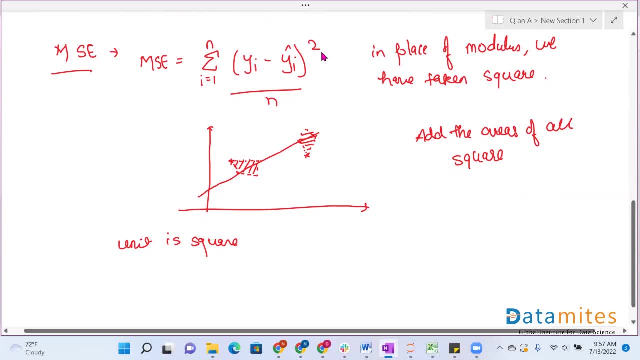 this is the unit of MSC. So this is the unit of MSC. So this is the unit of MSC. So this is square: okay, Because we are taking the square. So, for example, we have column y of price: okay, We are predicting price of some house okay, House okay. So we will. 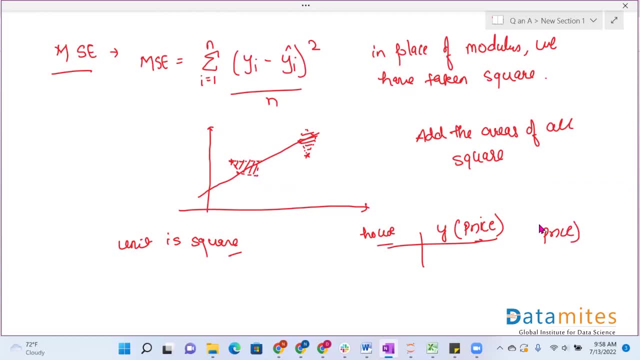 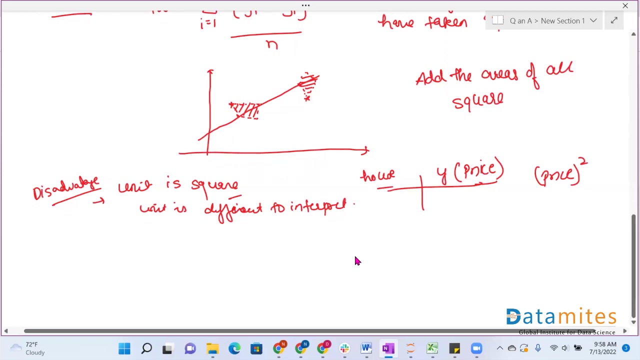 get the output as price square. So this is difficult to interpret, okay. So this advantage is that the unit of this is difficult to interpret- difficult to interpret, okay. And this is not good in case of outliers. This is not good in case of outliers, okay. 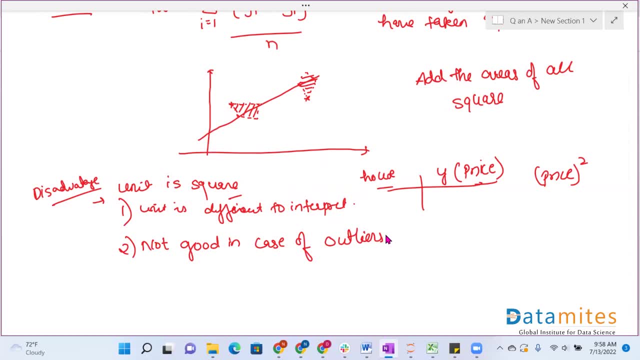 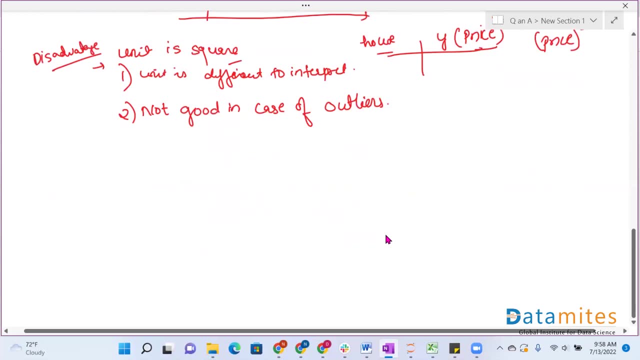 So we will move towards RMSC. okay, So we will move towards RMSC. third. type of RMSC, that is: root mean square error, root mean square error. okay, So here we have seen that the unit is not good in case of outliers. okay, So we will move towards RMSC third. 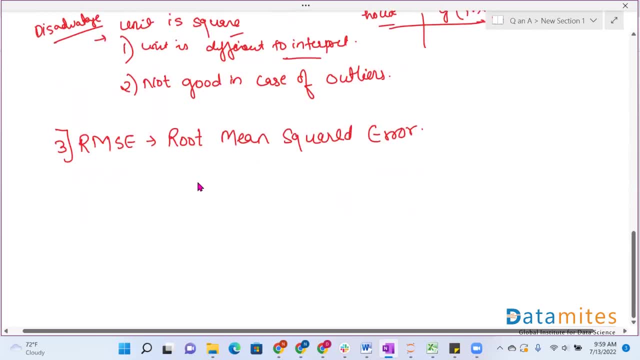 type of RMSC tomato, but not interpretable. But here we will take the root of this. So RMSC is given by under the root of MSE term. okay, So integration i equals to 1 to n yi minus yi hat square divided by n. So now the unit is same, But again the outlier problem. 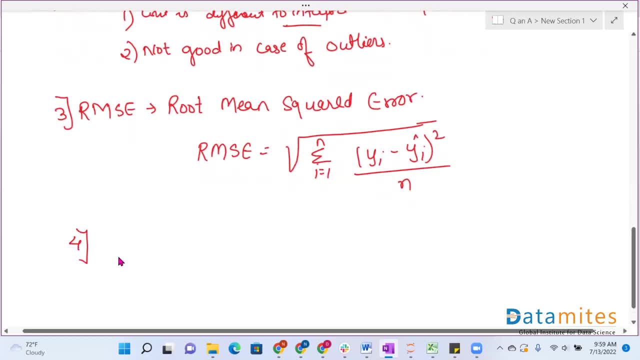 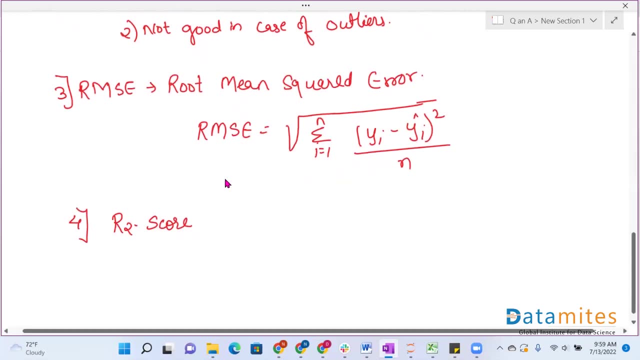 is not solved. okay, So we have next type of evaluation rightol further. Okay, So what we will do? we have matrices. that is R2 score, So this is also known as coefficient of determination. Okay, So we see that these three terms, that is, MAE, MSE and RMSE, will calculate the error. 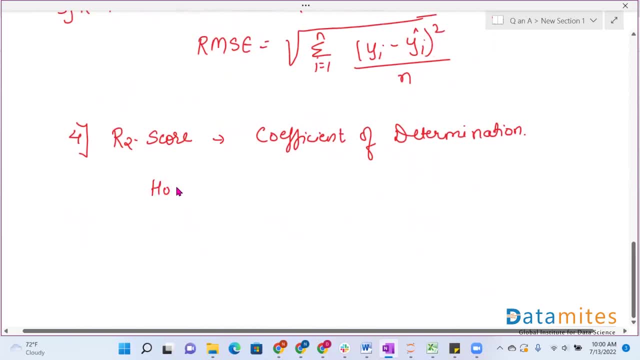 but R2 score will tell us how much good our model is. Okay, So this will tell us how much good our model is. This is also known as goodness of fit. This is also known as goodness of fit, Okay, So the formula for R2 score is given by: 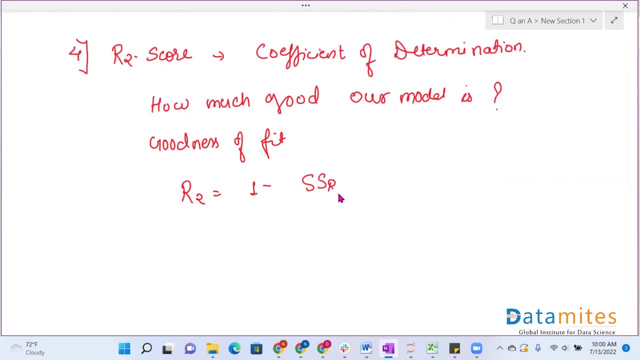 1 minus SSR divided by SSM: Okay. So SSR stands for sum of squared error in regression line: Okay, And SSM stands for sum of squared error, sum of squared errors in mean line- Okay. So what actually R2 score does? 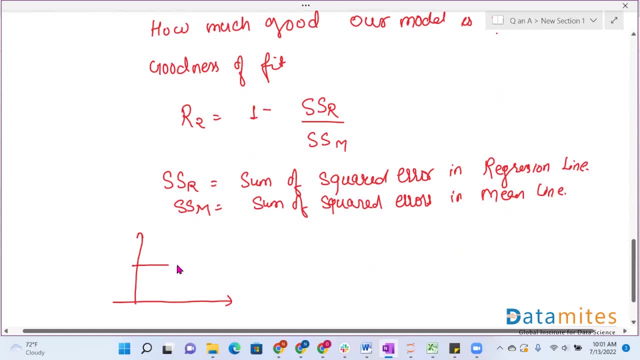 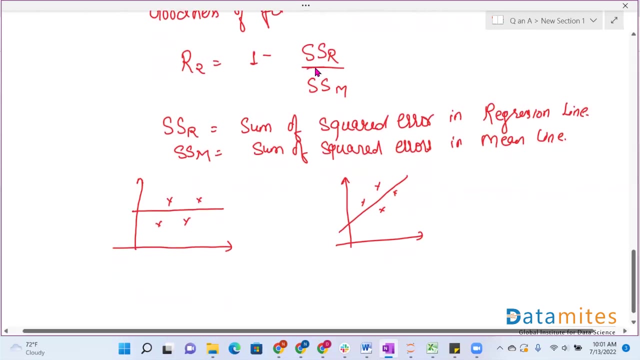 It will take for all data points. it will take one mean line and it will take the regression line. Okay, What is our best fit line? So it will take the regression line and it will take the mean line. Okay, So it will take. calculate the error squared of error for. 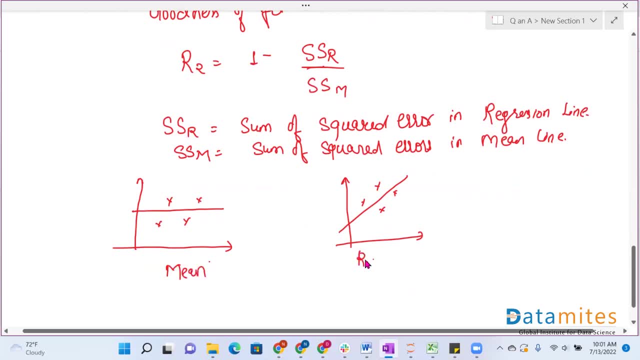 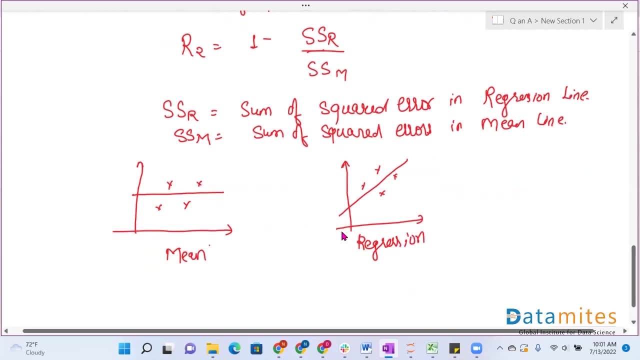 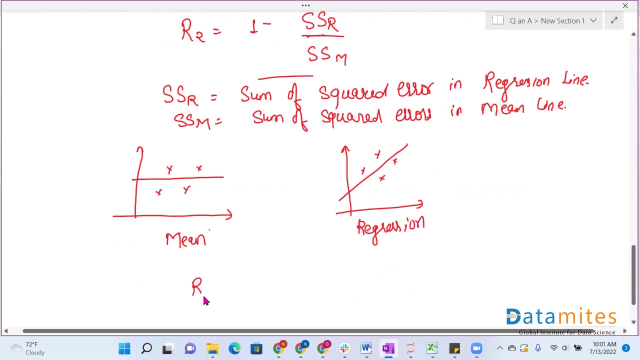 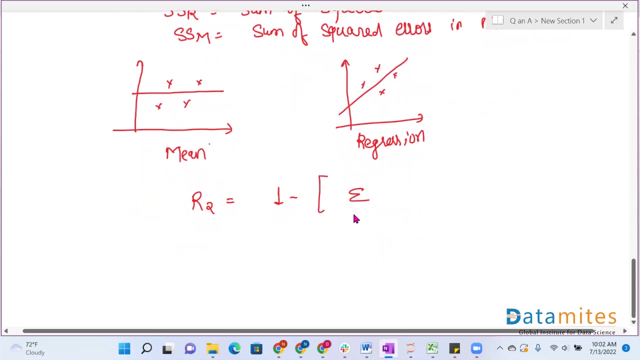 both the cases, for mean case and for regression line also. Okay. So it will take the squared errors for both the cases. Okay, And it will compare it. So this formula, so this formula now can be written as: R2 equals to 1 minus 1 minus summation, i equals to 1 to n yi minus yi. 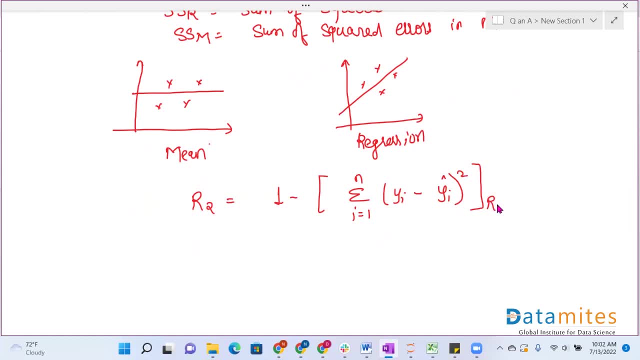 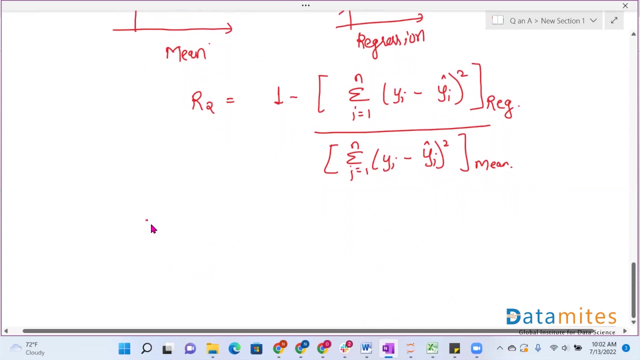 hat that is predicted square for regression line divided by i equals to 1 to n yi minus yi predicted for mean line. Okay, Okay. So this is the formula for R2 score. So the value of R2 score, that is, range of R2 score, can be varied from minus 1,. 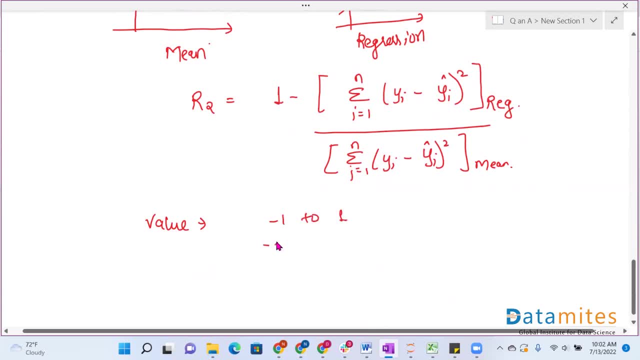 to 1.. Usually it is between 0 to 1.. If it is minus 1, it is worst model. The model is not performing good. If it is near to 1, we can say that the model is performing good. 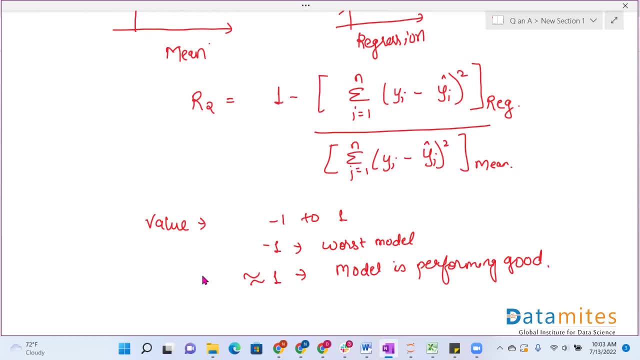 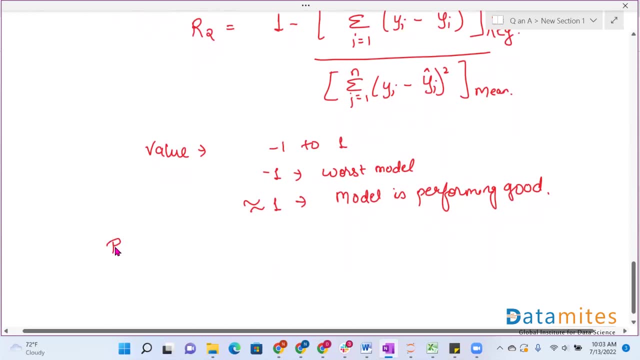 Okay. So now, if we see that, if we see that the what R2 score actually tells us, Okay So, let us take the example: R2 equals to 0.80.. Okay, So the value of R2 score is 0.8.. Okay. 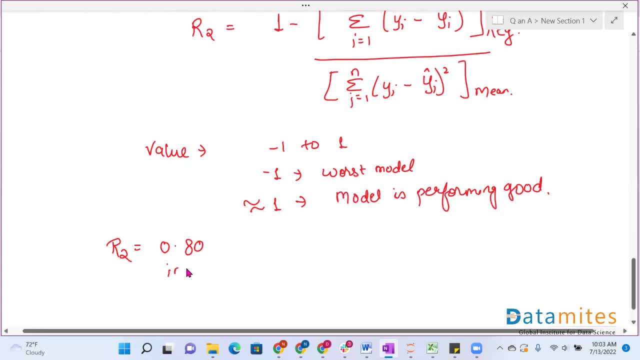 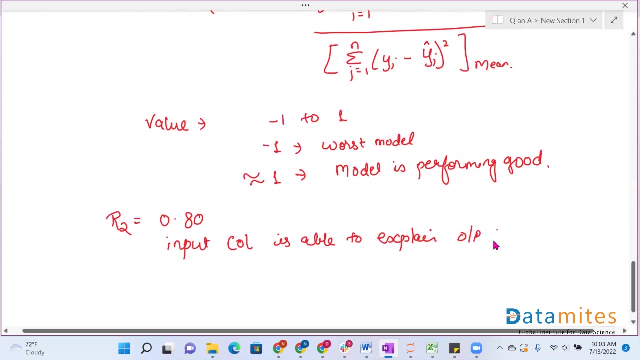 So what this interpret that how much input column, how much input column is able to explain? about the output column? Okay, About output column. Or we can say that input column is able to explain 80% of variance in output column. that is, input column is able to explain. 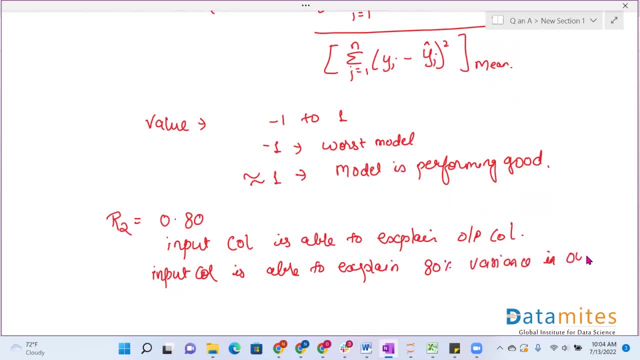 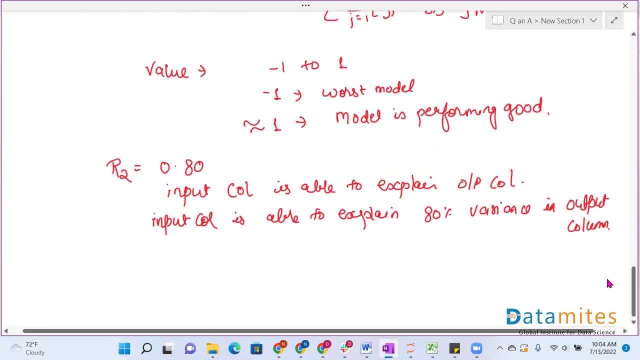 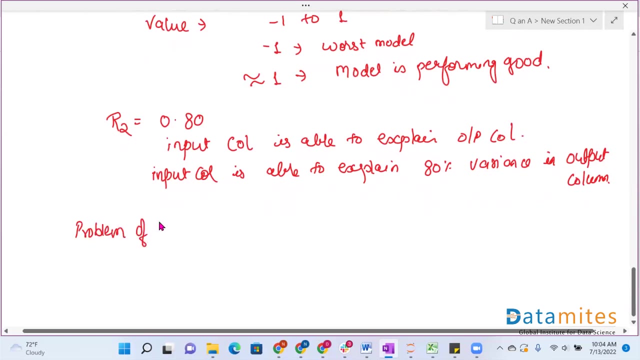 80% variance in output column. okay, so this is given by r2 score. but again, there is a problem with r2 score. that is a disadvantage of r2 score. okay, so the disadvantage is it behaves sometimes same when a irrelevant column is added. okay, so, for example, for example, i have a data set in which i have cgpa.